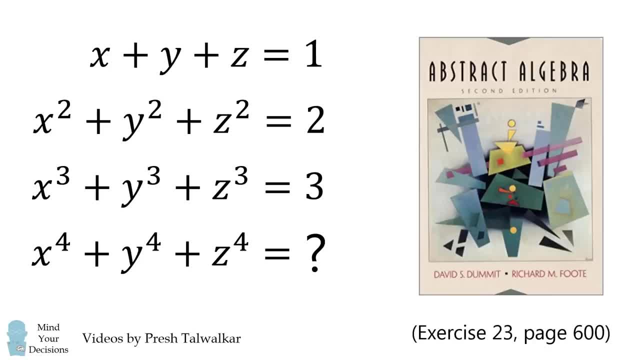 You could solve the sum of the fourth powers and the sum of the fifth powers using high school algebra and clever tricks. It's not easy, but it is possible. In this video, I'm going to show you a systematic approach to solving these problems. 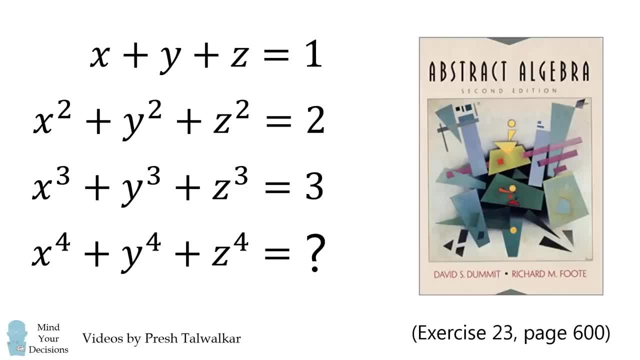 And it will involve a little bit of build up because we're going to study some university level mathematical topics, But I think it will be worth it. Pause the video If you'd like to give these problems a try and when you're ready. 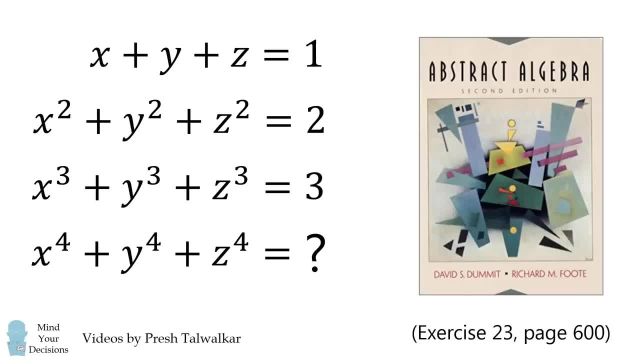 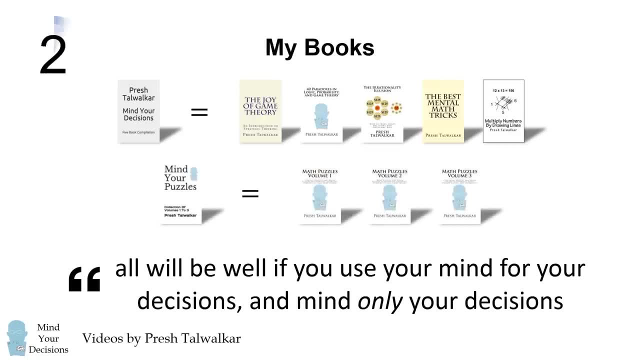 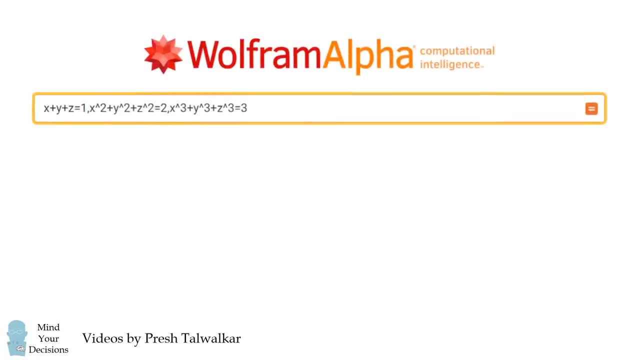 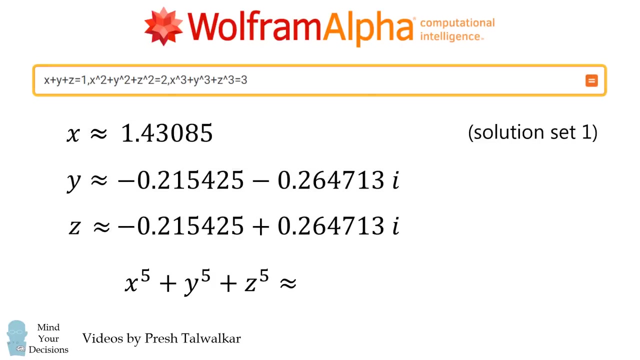 keep watching to learn how to solve these problems. We'll get started with the numerical approach. If we input these equations into Wolfram Alpha, we'll get approximate values for x, y and z. We can substitute that in to get an approximate value of x, y and z. 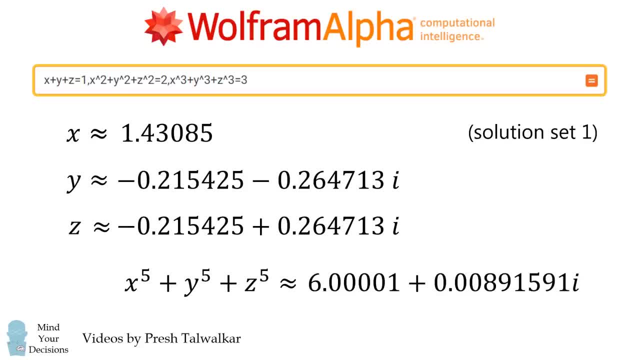 For the sum of the fifth powers. It appears to be a complex number, But we might just take a guess that this is a real number and it's equal to six. In fact, this is the actual answer, which we'll prove later in the video. 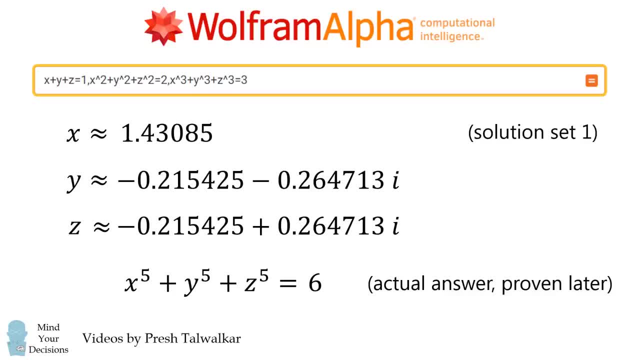 But there's something interesting: when you take a numerical approach, You get more than one solution set of x, y and z. You actually get six different solution sets. by permuting the values for x, y and z, In total there will be three factorial, which equals six solution sets. 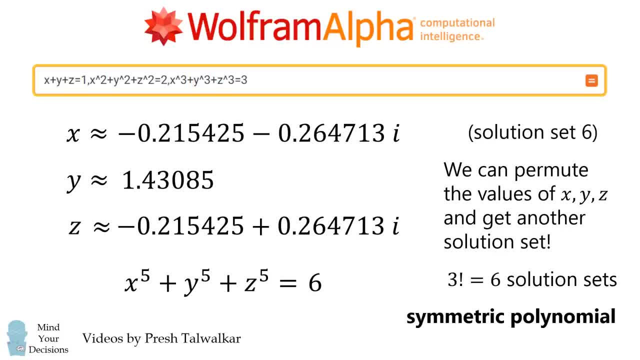 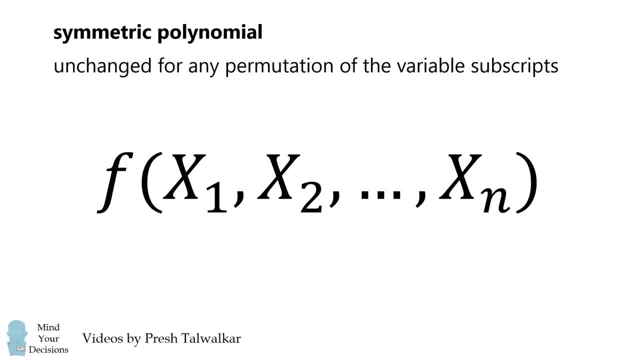 The reason for this symmetry is we're dealing with symmetric polynomials. A symmetric polynomial is one in which it's unchanged for any permutation of the variable subscripts. If we exchange one and two, we would have to get exactly the same polynomial. If we do a more complicated permutation, we would also have to get exactly the same polynomial. 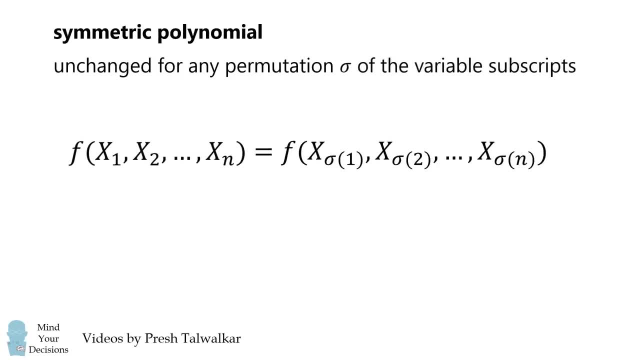 In general, this polynomial has to be the same for any permutation sigma of the variable subscripts. So let's take a look at a concrete example. Consider the polynomial x1 plus x2.. It's unchanged for the identity permutation, which does nothing. 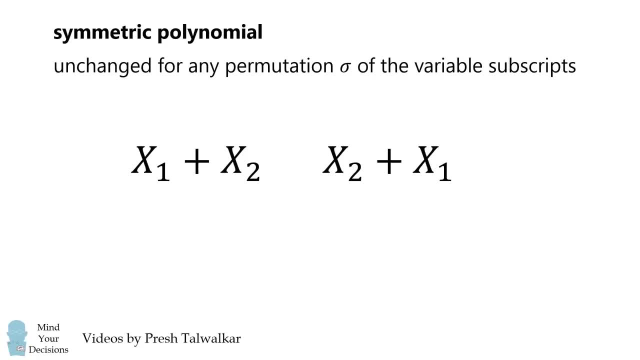 And it's also unchanged for the other permutation that transposes one and two. These two polynomials are always equal to each other, and therefore x1 plus x2 is a symmetric polynomial. On the other hand, x1 minus x2 is not symmetric. 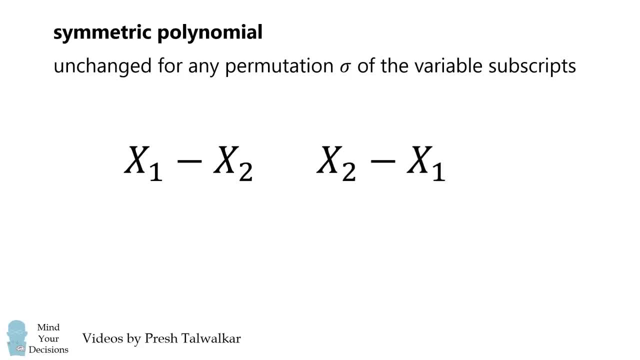 While it's unchanged for the identity permutation, it is changed if we transpose one and two. In general, x1 minus x2 is not equal to x2 minus x1.. This is not a symmetric polynomial, But we can modify this to get a symmetric polynomial. 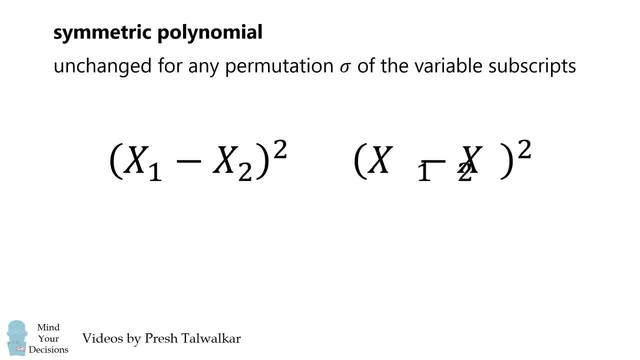 Imagine we square the polynomial. This will be a symmetric polynomial. I'll mention that What we're doing is an example of group theory, which is the study of such symmetries. I briefly introduced group theory in my video. Multiply by Lines: Group Theory. 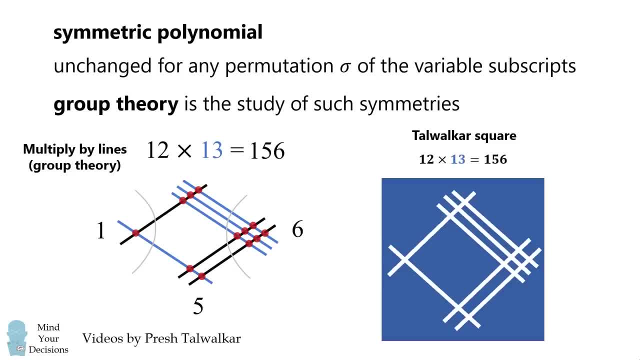 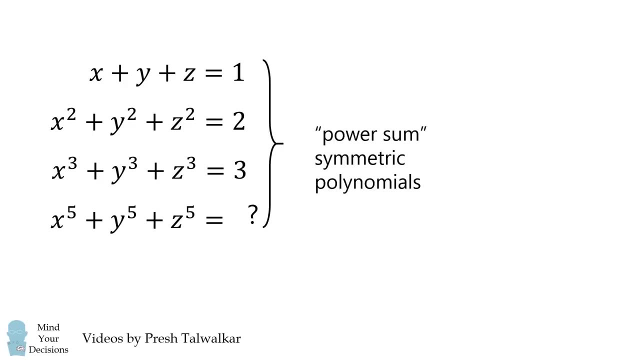 I showed that you could take the tall walker square diagram for an arithmetic problem and then exploit the symmetries of the square to solve new arithmetic problems. So how does that relate to our original problem? Well, these are a system of power-sum symmetric polynomials, or 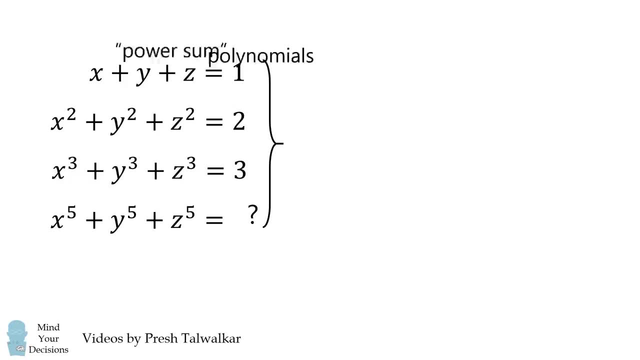 power-sum polynomials, for short. Each of these is a different power-sum polynomial and the degree refers to the exponent of the variables. Let me just put this in a little bit more formal notation. The kth degree power-sum polynomial for n variables will be the sum of the variables to the kth power. 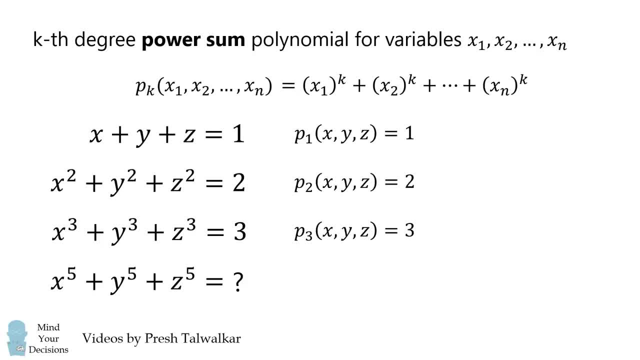 So we'll translate our equations into power-sum polynomial notation. We want to solve for p5.. Now, since we know we're dealing with three variables, we'll just abbreviate this by removing the x, y and z. So how can we solve for the value p5?? 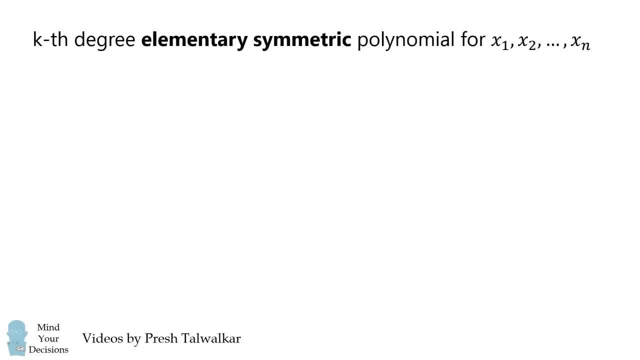 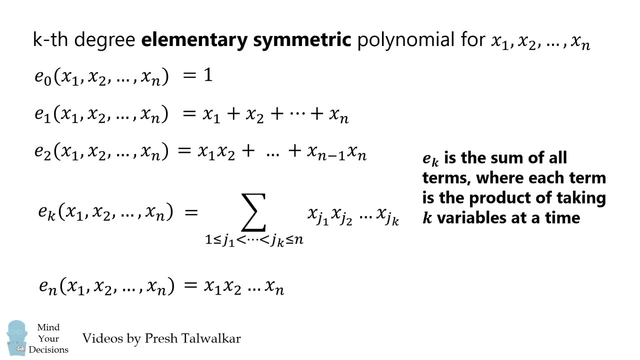 To do that, we'll need to study the elementary symmetric polynomials. These are the building blocks for all symmetric polynomials. So let me just show you the formal definition and then I'll give you some intuition. ek will be the sum of all terms, where each term is the product of taking k variables at a time. 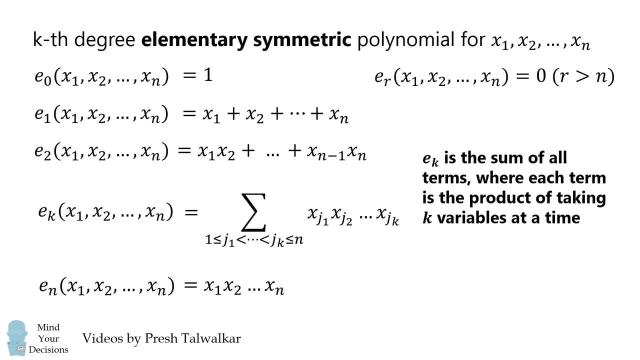 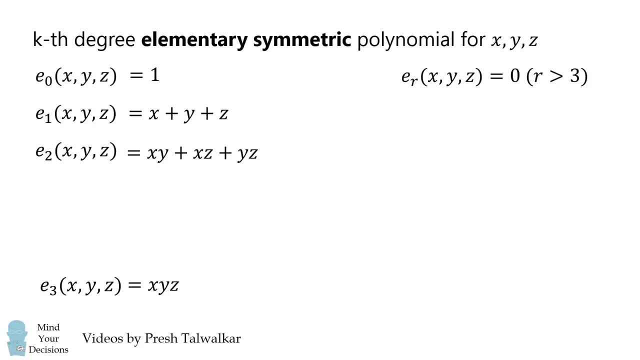 And if we have more than n, so e of r for r greater than n it'll be equal to zero. In our problem we have three variables: x, y and z. These are the elementary symmetric polynomials. Since we're dealing with x, y and z, I'll just abbreviate this. 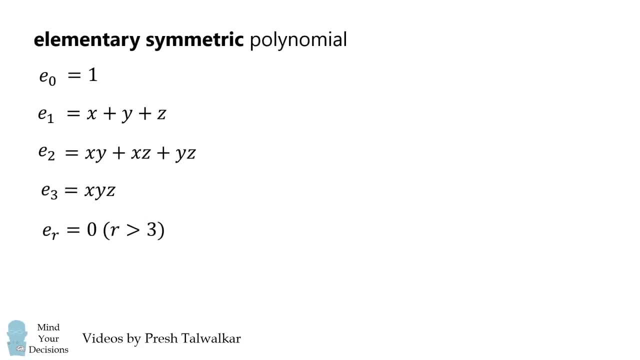 And now we're going to take these elementary symmetric polynomials and relate it to the power-sums. To do that, we'll start all over. Consider a polynomial of degree n as follows. They'll be in the variable t. This will have n roots over the complex numbers and we'll label them as x1 to xn. 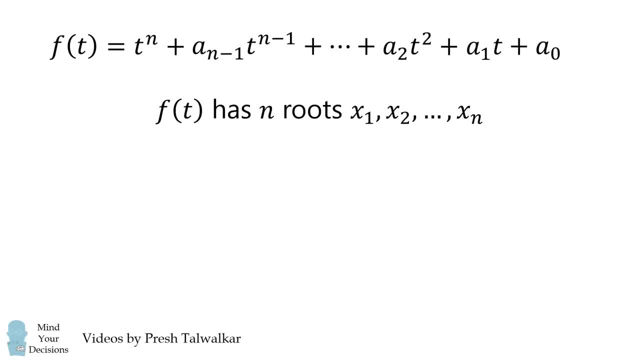 Some of the roots may be equal to each other, but that doesn't matter. It'll have a total of n roots. Therefore, we can factor the polynomial as follows: It'll be the product of these linear terms. We can now compare these two versions of the polynomial. 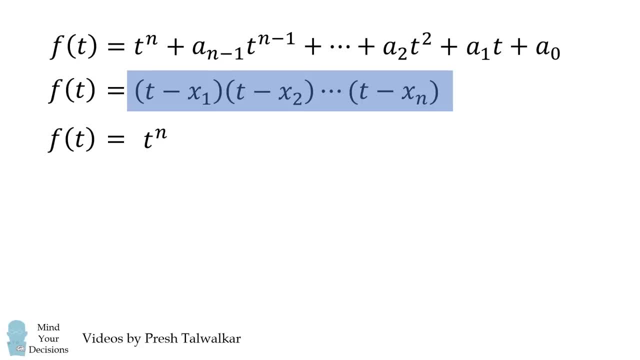 So what happens when we expand this polynomial? Well, the leading term will be t to the power of n. We then have negative e1 multiplied by 1.. And we multiply by t to the power of n-1.. The coefficient on the second term will be negative. the sum of the roots. 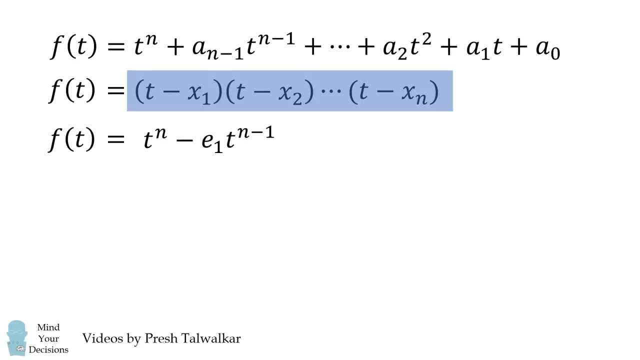 And that's something you might have learned in school, but this is where it comes from Now. the next term will also have a coefficient, that's an elementary symmetric polynomial, And this will actually continue in an alternating sum. Now what can we do here? 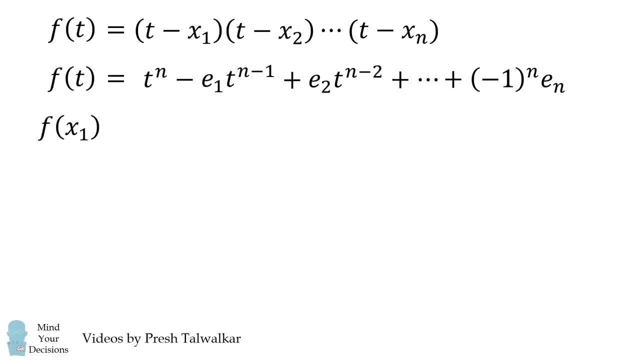 We'll make some substitutions. Suppose we have f of x1. Well, in the first equation we know that this factor will cancel out to be 0. Because x1 is a root. Therefore we know this is equal to 0.. 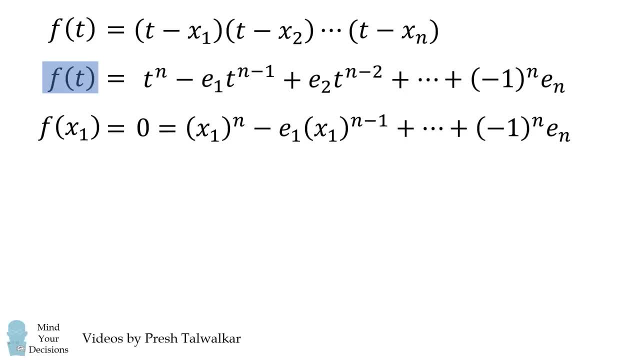 But we can substitute it into our second equation And we'll get the following expression. We can do this for all of the n roots. On the one hand it'll be equal to 0. And on the other hand we'll get an expression. 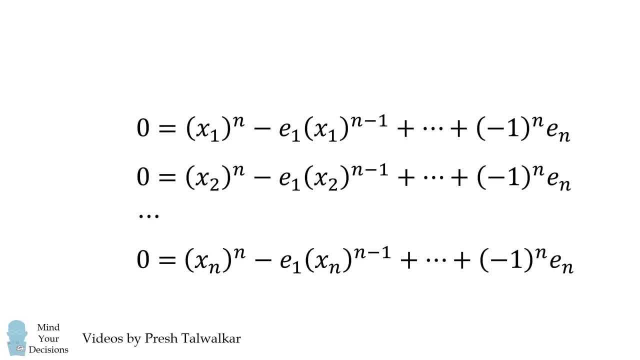 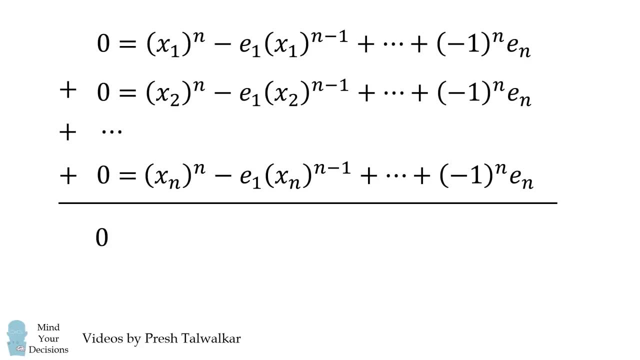 So when we do that, we get a system of n equations And we can do something interesting: We can sum these equations together. The left-hand side will be equal to 0.. Now what happens on the right-hand side? We'll sum column by column. 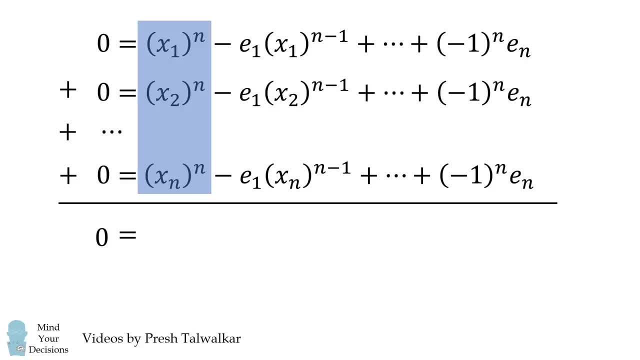 The first column will be the sum of these n variables to the nth power. In other words, this is Pn. It's a power-sum polynomial as the leading term. This pattern will continue for the rest of these sums. We're going to get power-sum polynomials. 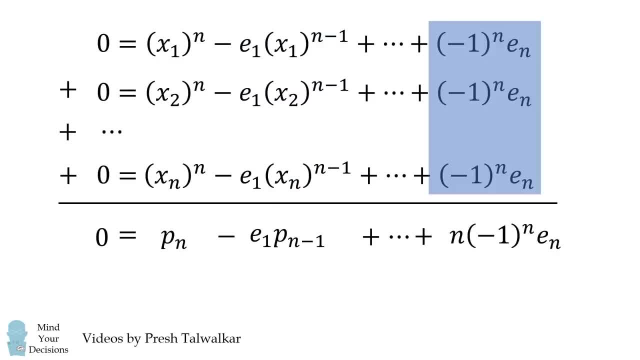 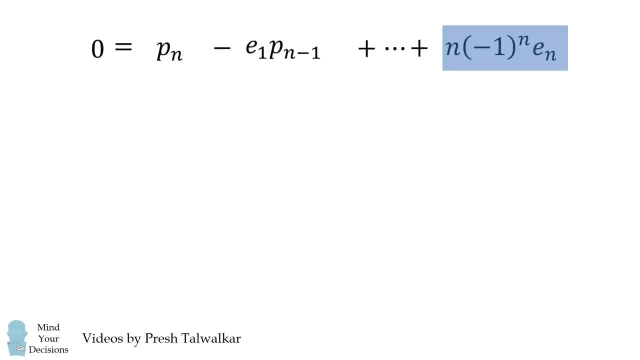 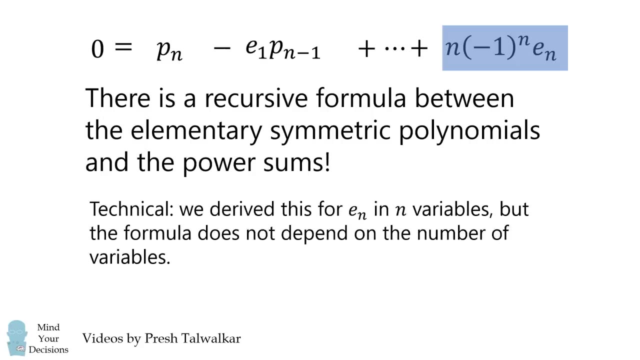 All the way until the very end where we get n times negative 1 to the power of n En. Now this formula right here is interesting. It relates the elementary symmetric polynomials to the other polynomials and the power-sums. Now technically we derive this for En in n variables. 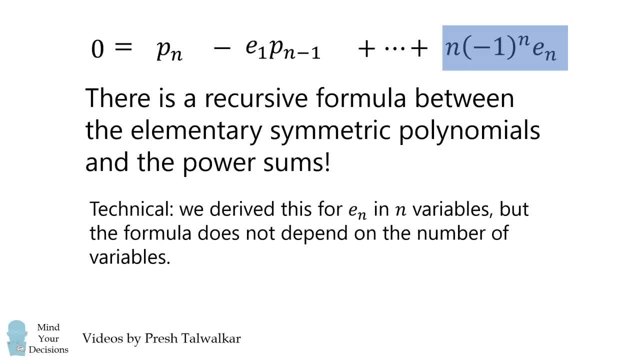 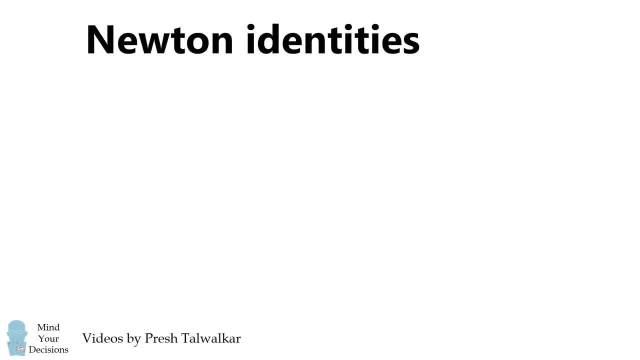 but this formula actually doesn't depend on the number of variables, And I'm going to present it in another way which will be useful to solve our problem. So these are often called the Newton identities, But they were discovered in 1629 by Einstein. 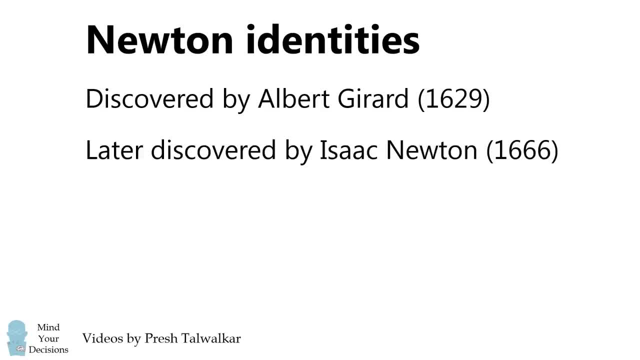 Albert Girard, And then it was later discovered by Newton in 1666.. Some people call them the Newton-Girard identities, But, at Mind Your Decisions, we respect mathematical history and believe it would be more correct to call them the Girard-Newton identities. 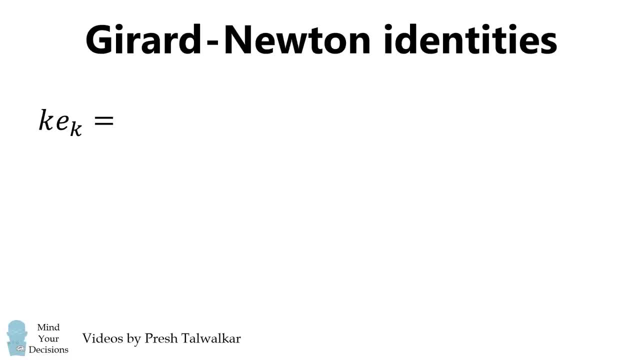 So here are the identities: k multiplied by Ek is equal to Ek minus 1, multiplied by P1 minus Ek minus 2 multiplied by P2 plus so on, in an alternating sum, All the way to negative. 1 raised to the power of k minus 1, E0 multiplied by Pk. 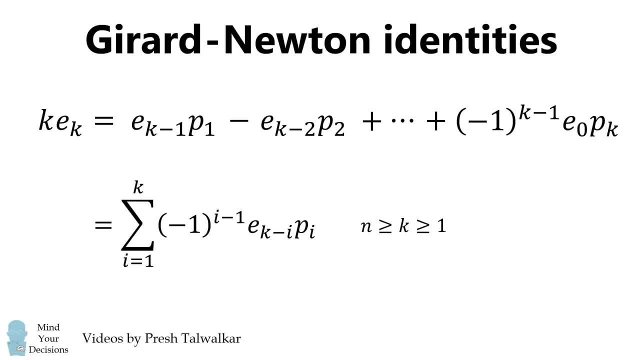 This is what the formula looks like in sigma notation. So here are some tricks to remember this formula. It starts out with Ek minus 1 multiplied by P1.. This will always be true. We then have an alternating sum And, finally, each term will have the following form: 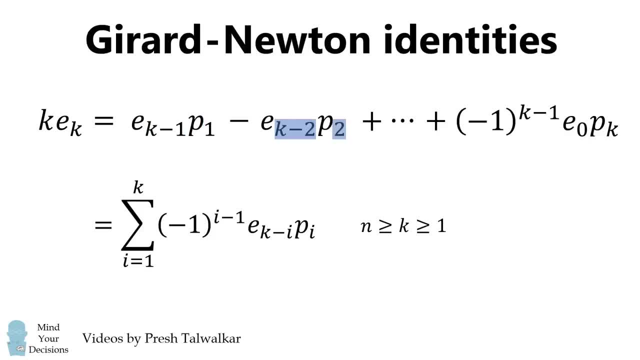 The elementary symmetric polynomials will decrease, while the power-sum polynomials will increase, And the sum of the indices will always be equal to k in each of these terms, And that goes all the way to the very end. So we'll use these identities to solve our problem. 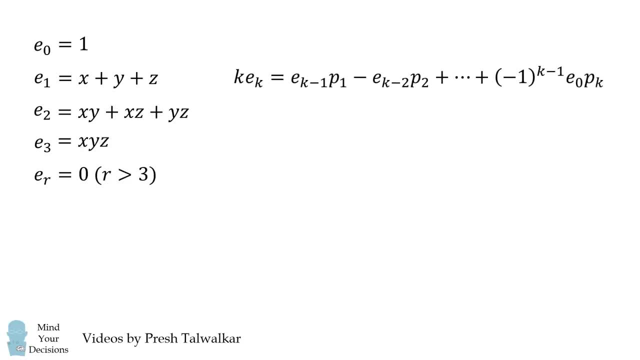 To recall, these are the elementary symmetric polynomials related to x, y and z, And these are the power-sum polynomials that we were given and the values of them. So we'll get started. that P1 equals 1, and that's exactly E1.. 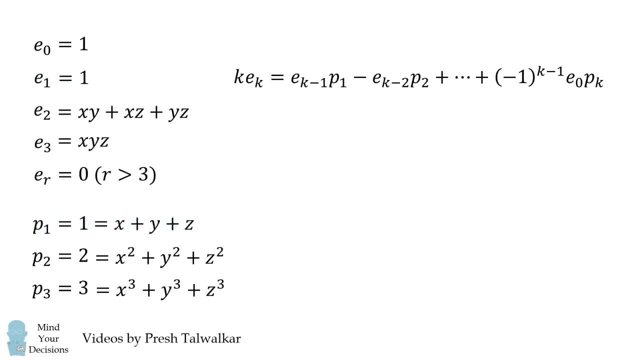 Therefore, E1 is equal to 1.. Now let's solve for E2.. E2 is equal to 1.. 2 multiplied by P1 equals 1.. 3 multiplied by E2 equals E1P1 minus E0P2.. 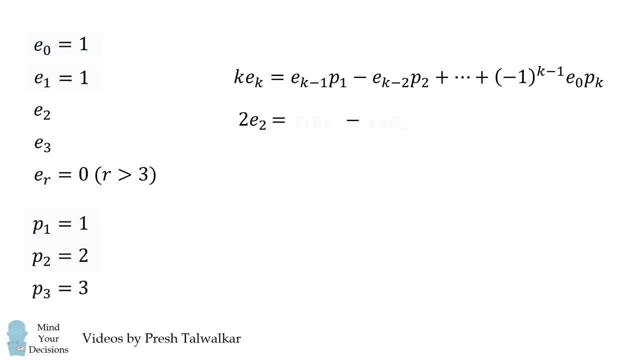 We have the values for all of these except E2.. So we'll substitute in and simplify and we can solve that E2 is equal to negative 0.5.. We now will solve for E3.. 3 multiplied by E3 will be equal to E2P1 minus E1P2 plus E0P3. 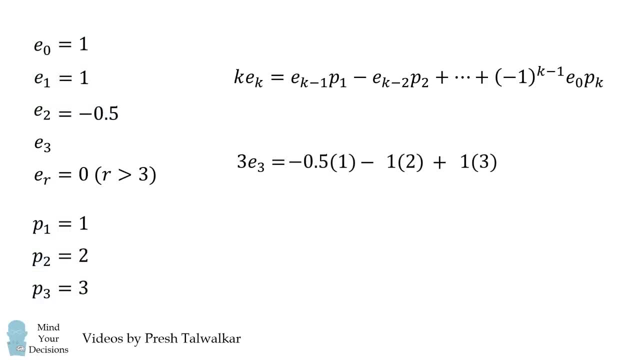 We substitute in the values we've derived And the only thing that remains will be: 3 times E3 will be equal to 0.5.. Therefore, E3 equals 1 over 6.. Now consider 4 times E4. This will be equal to E3P1 minus E2P2 plus E1P3 minus E0P4.. 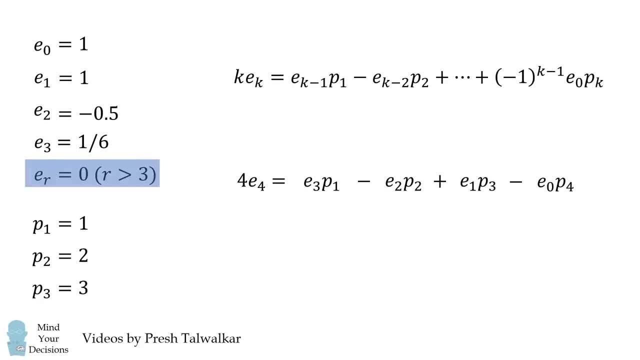 What is E4?? Well, 4 is greater than 3.. So the answer is E2P2.. So the elementary symmetric polynomial will be equal to 0.. This term will vanish. We then substitute in values for the things we've already derived. 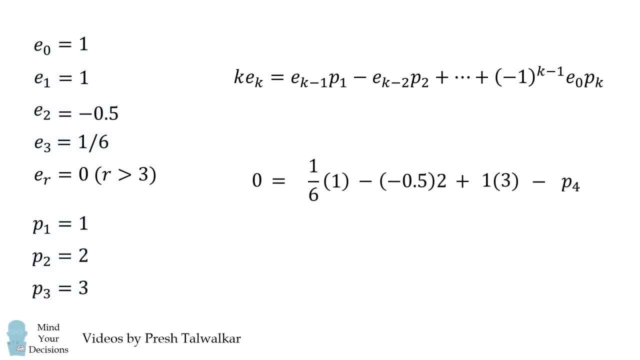 The only unknown in this equation is P4. And we have a linear equation which we can solve for P4. It equals 25 over 6.. And recall, P4 is the power sum polynomial, the sum of the fourth powers. So this is one part of the problem we've already solved just by going through this formula. 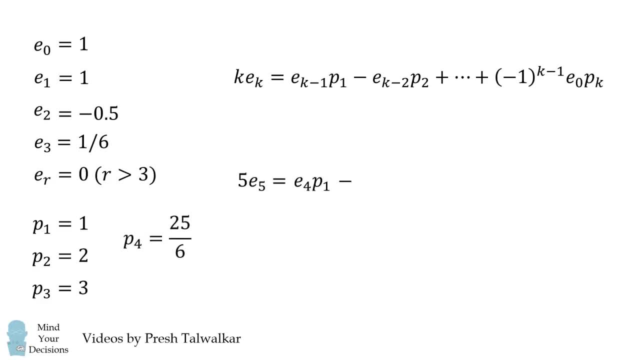 Now let's look at 5 times E5. It'll be the following expression: And E of 5 and E of 4 will be equal to 0, because 5 and 4 are greater than 3.. So these terms will vanish. 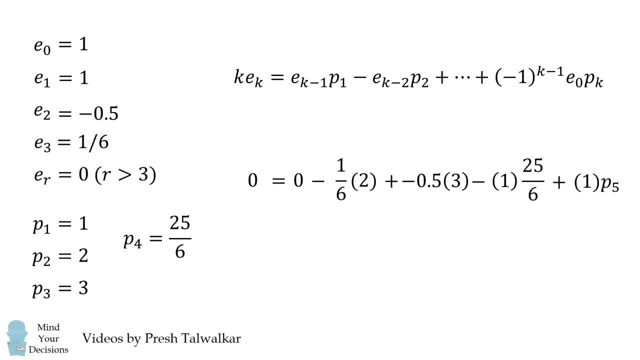 We then substitute in values we've derived, And the only unknown is P5.. We'll solve for P5 and we get the value of 6. And that's the answer to our problem. This is the sum of the fifth powers And we've derived it using the other elementary symmetric polynomials. 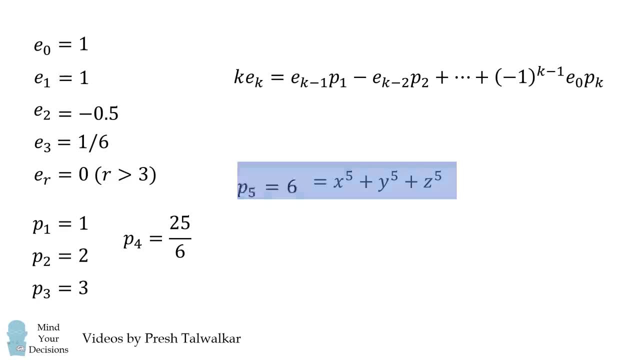 and the other power sums. This is incredible. Now I have a challenge for you. Try to solve for the sum of the sixth powers. Furthermore, prove that the sum of the nth powers is rational for every positive integer n. Thanks for making Mind Your Decisions. one of the best channels on YouTube. 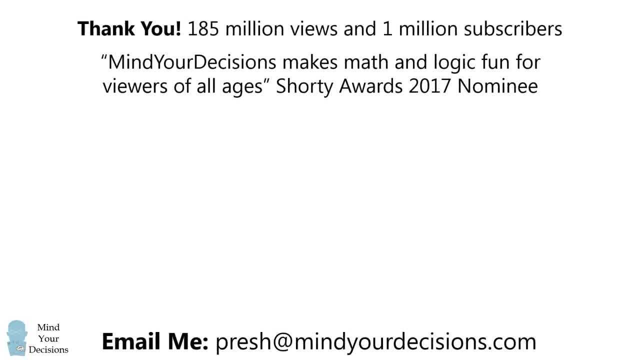 As always, thanks for watching And thanks for your support.